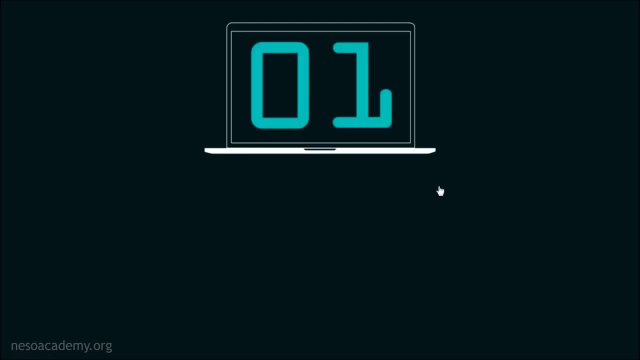 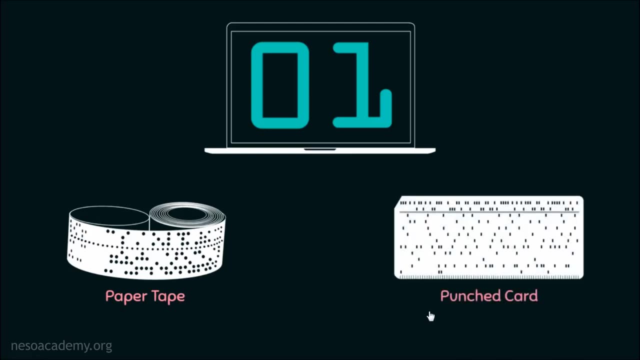 and ones. Therefore, in early days of computation, instructions to a computer were given using perforated paper tapes and punch cards. In these, the presence of a hole is a representation of zero and absence means one. Now, writing down instructions in the form of ones and 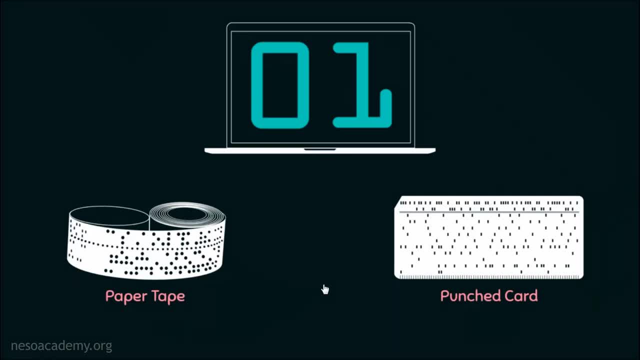 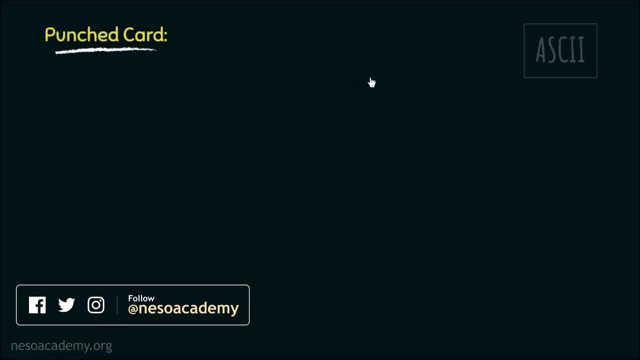 zeros is pretty hectic. Let me show you how Let's take this word punched card. If we convert this into its equivalent binary using ASCII standard. now, ASCII stands for American Standard Code for Information Interchange. it becomes this: Now, this is the format which computers can process directly, But for us it is almost. 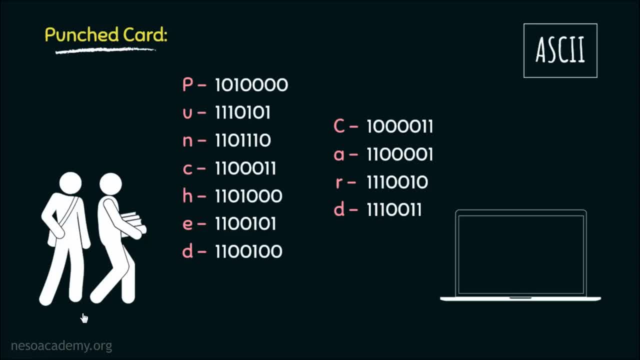 impossible. Even if it becomes possible for any human to encode instructions like this, it is undoubtedly time consuming. Now think about the situation carefully. At one hand, we have a machine that has immense potential. We can employ it to solve many of our problems. 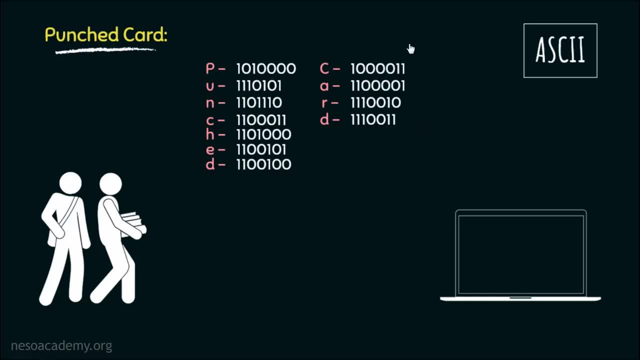 But, on the other hand, we are facing an awful lot of trouble while communicating with it. So what is the solution? Since we are facing a communication barrier, we need language translator. In simpler terms, we will say: punch cards and the middleman. that is the. 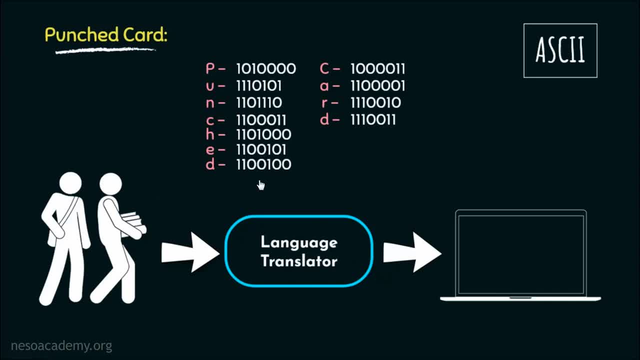 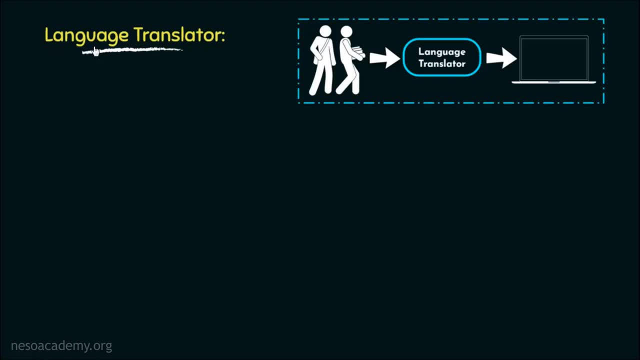 language translator will convert that into the strings of ones and zeros. Over the time, computer scientists came up with various language translators. The first one was the assembler Debut. in the late 19th century the assembler was called the assembler. The assembler was. 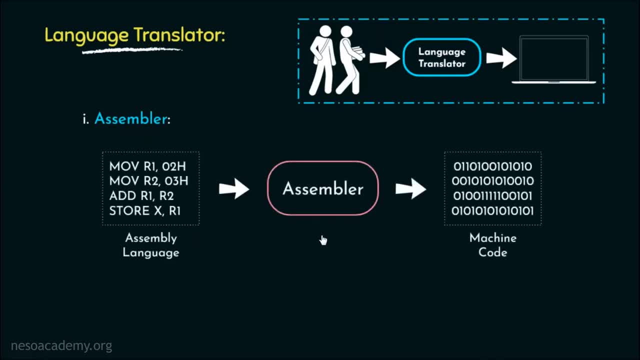 used to translate the code of the computer into the machine code. So the assembler was used to translate the code of the computer into the machine code. In the late 1940s these language translators could translate assembly language into its machine code, that is, strings of ones and zeros. 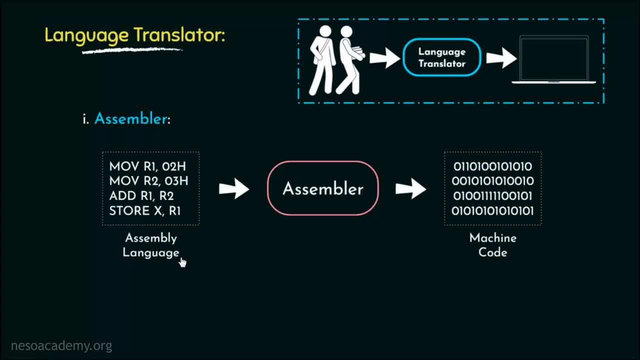 Now, assembly language has a very strong correspondence between the instructions of it and the architectural specification of the computer. That means, in order to write instructions for the computer in assembly language, the coder needs to have a proper knowledge about the computer's architecture first. It seems tedious too, doesn't it? 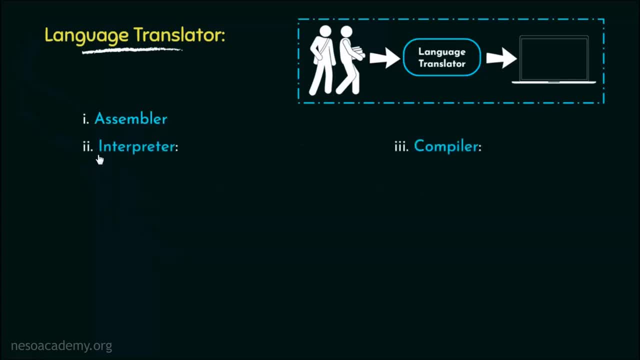 So in the 50s two new language translators- the interpreter and the compiler- came into picture. PHP, Ruby, Python, JavaScript are some examples of interpreted languages. That is when we write programs in these. the respective interpreters run through the programs one line. 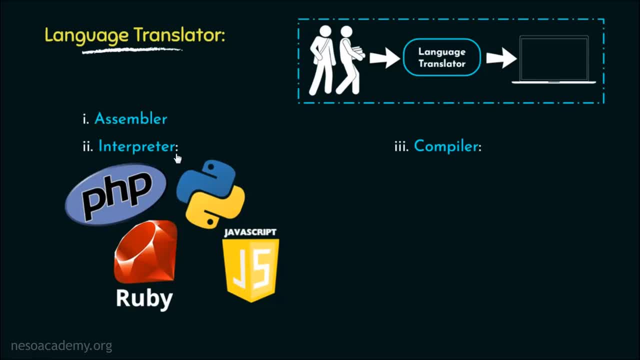 at a time, And so the compiler will write the programs one line at a time, And so the compiler will write the programs one line at a time And finally convert the programs into machine codes. On the other hand, C, C++, Erlang, etc are some common examples of purely 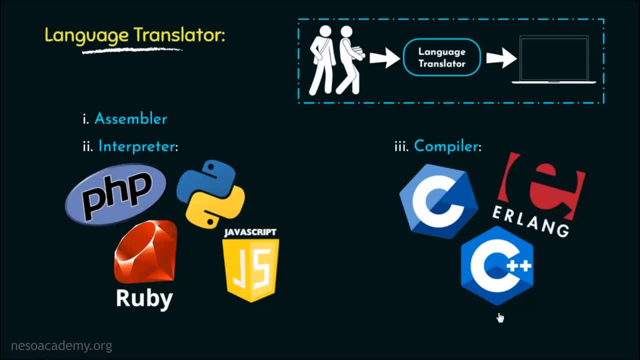 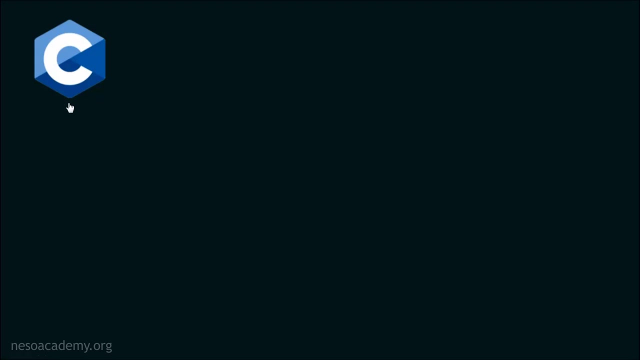 compiled languages, That is, programs written in. these are converted directly to the machine codes. Compilers tend to be faster and more efficient than interpreters, So this is how compilers came into picture. Now, many of us know about the C programming language right, Although nowadays it is. 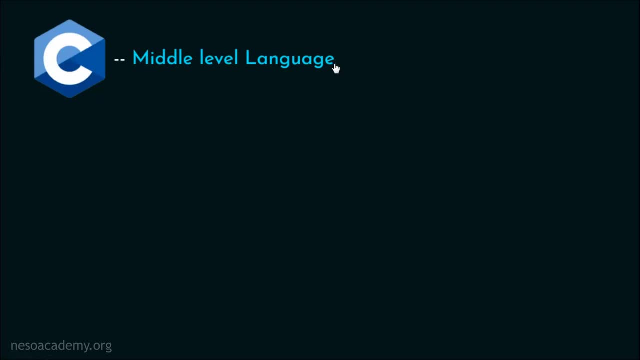 classified as a middle level language because of various features like direct memory, access through pointers, bit manipulation using bitwise operators and the ability to embed assembly code within C programs. However, originally it was classified as high level language because, syntactically, C codes are not the same as C programming languages. 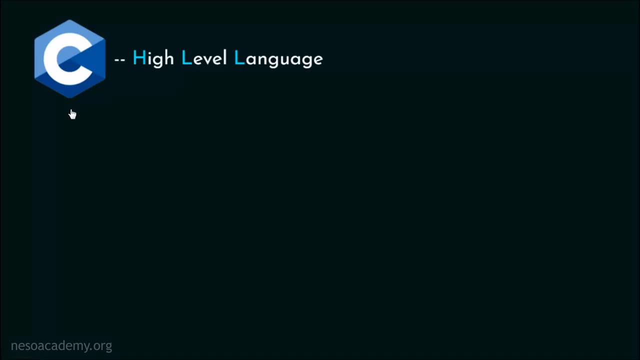 So the C programming language is a middle level language. However, it is classified as the inside theme of every language and too sevaray programming language. Now, a lot of language depends on C programming, So let us first compare how this programming code is structured. 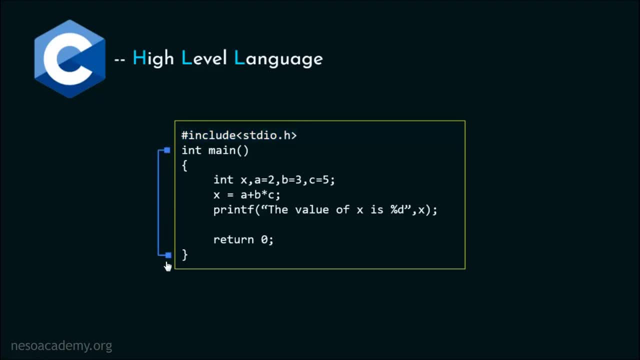 It is a very basic programming. code is int. Now here we have four integer variables: x, a, b and c. Now, apart from x, a has been initialized with the value 2,, b with 3, and c is initialized with 5.. Coming to the next statement, 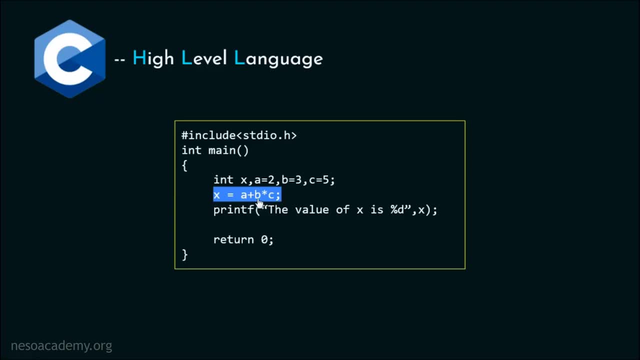 it's actually an arithmetic expression. Here first b is multiplied with c, and thereafter the result is added with a and finally it is assigned to the variable x. And here we are printing the calculated value of x on the screen using this printf function. By the way, we have 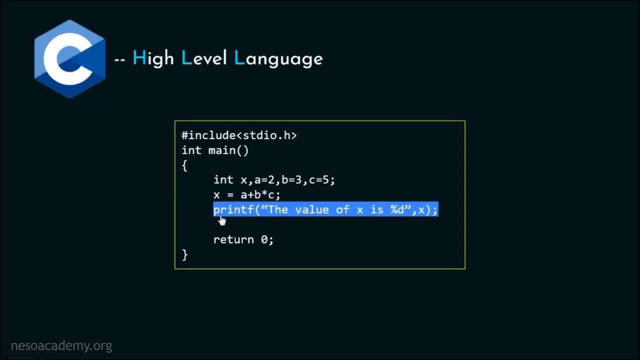 to include the standard input output header file because we are using the printf function. If we don't want to print the value of x on the screen, we need not write this line Now. finally, here we are returning 0, because this function main is not supposed to return anything under error-free execution. 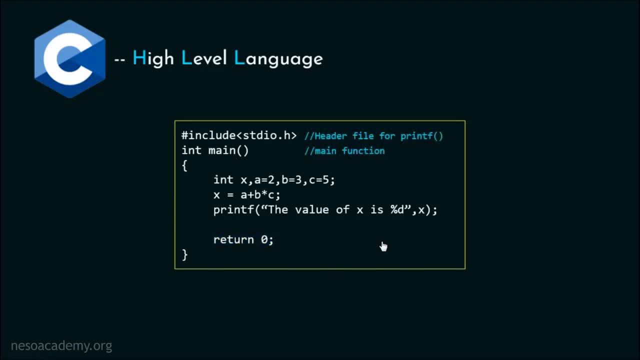 Now, if you observe, this piece of code is close to English. right Header file is being included using hash. include preprocessor directive. The main function is actually the main part of the code. Integers are given the data type named int and finally, printing is happening through the printf. 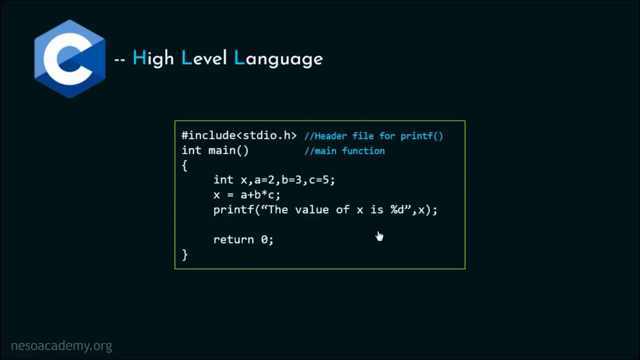 function. So it is in human readable form, but the machine is not able to read it. So we are printing the value of x on the screen using the printf function. Now, the machine cannot understand it. We usually call it the source code or high level language code, And the job of the language translator is to convert this high level. 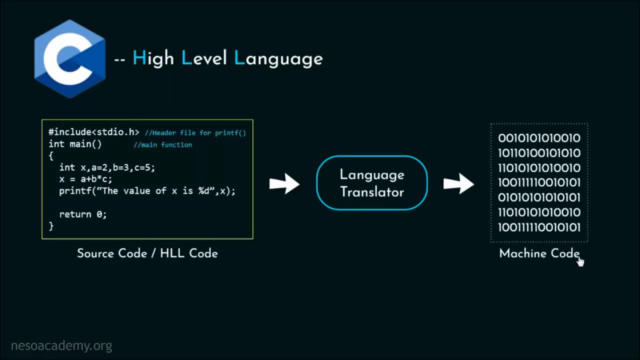 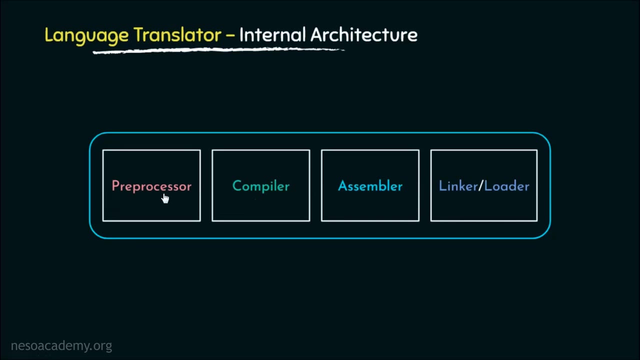 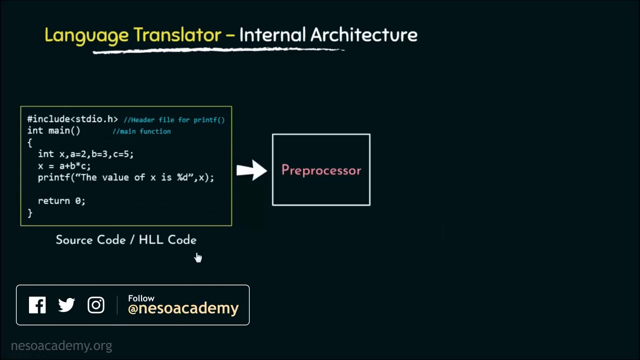 language code into executable machine code. Now let me walk you through the internal architecture of the language translator. Specifically for C language, the language translator has four different phases. The first one is the preprocessor. This preprocessor will resolve all the preprocessor directives As for this particular code. 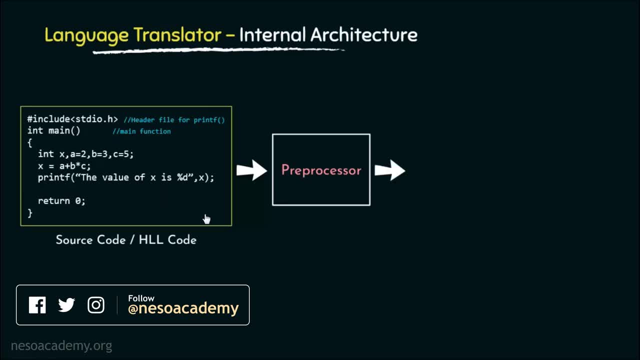 reading the hash include preprocessor directive. it will append the standard input output header file to the high level language code, removing the preprocessor directive. Also, it will remove all the comments. So now the high level language becomes a pure high level language. The next one: 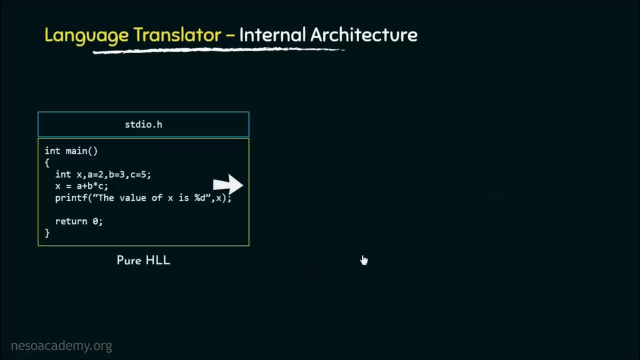 is the compiler. This phase will generate the input output header file to the high level language code. The compiler must be confirm, while the cuerpie allows the Hetero edge to render the Lukas as the high level template of any two Scikit thing. 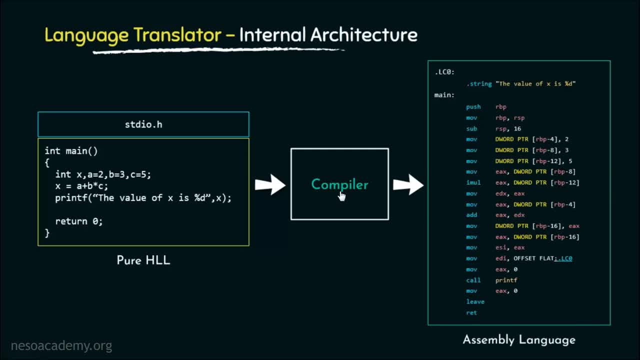 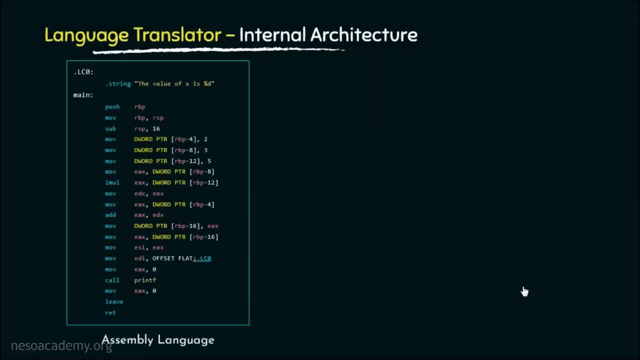 And let's talk about the personally. This is the assembly code and its years, before I ugly text here. Do you know? separate assembly, Python center pol出, where P are per Orございます, As you can see here, as simple As you can see here. this is the assembly code of this Pure high level language code and the compiler is responsible for this translation there. after this assembler will generated the relocatable machine code. now, relocatable machine code is actually streams of ones and zeroes, which is actually the machine code. however, this is relocated also kill, cut, taken from the system. now, if we want our English, 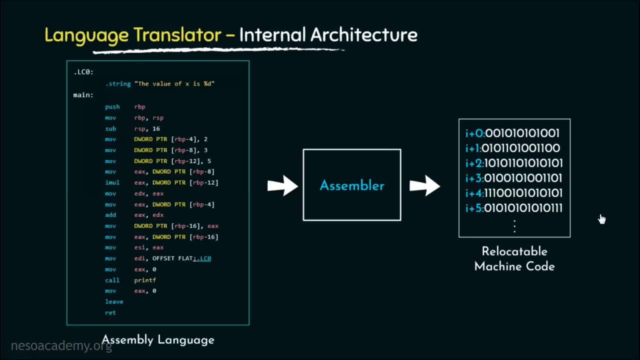 relocatable. okay, let me put it to you this way: a program turns into a process during execution, right, and only during execution. it is allocated to the main memory. so before execution, we cannot know where exactly in the RAM the process will be located. so, for that time being the sequence of the machine code: 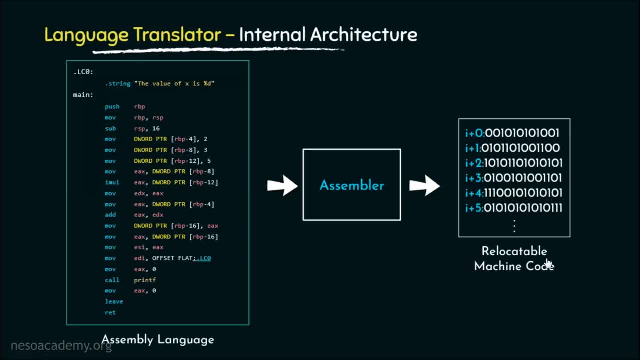 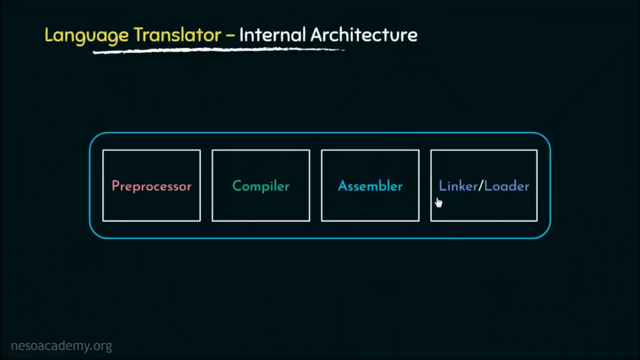 instructions is given a relocatable address. as you can see here, the first instruction has the address I plus 0, and then the successive ones have I plus 1, I plus 2 and so on. basically these are sequential. here, I is the variable which signifies the relocate ability. finally, the last one, that is the linker. 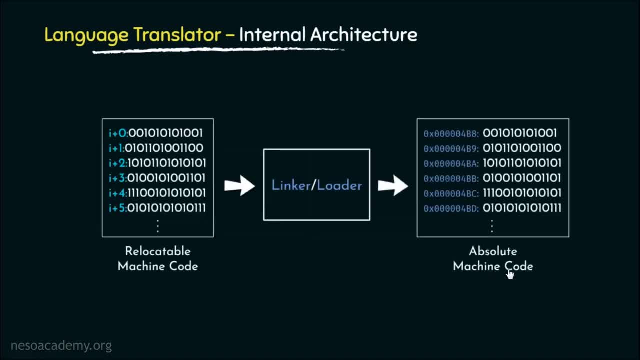 and loader. these generate the absolute machine code. that is actually the executable machine code. this one is basically the process which has the address i plus 0, and then the successive ones have i plus 1. i plus 2 has been loaded into the RAM and is ready for execution. see, these are some. 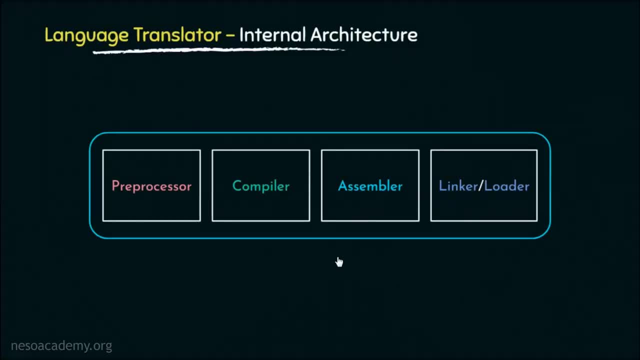 sequential absolute addresses. so this is the underlying architecture of the C language translator. now, from all these, the second one, that is, the compiler, is what we are going to focus on in this compiler design course. now coming to compilers, it has six different phases. these are: lexical analysis, syntax. 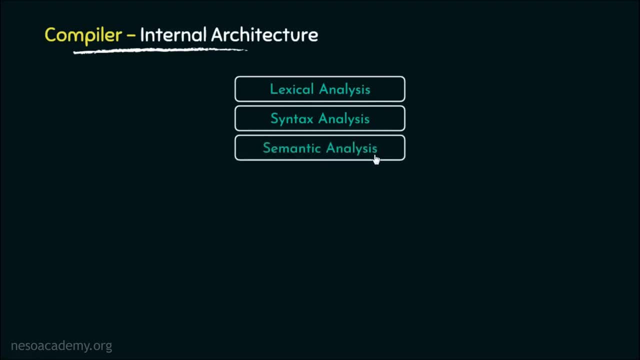 analysis, then the semantic analysis phase, after that the intermediate code generation phase, the code optimization phase and, last but not least, the target code generation phase. now, face wise, the first three phases are called analysis phase, whereas the remaining three, unknown, as synthesis face. however, from a software's perspective, the first four phases, that is, the 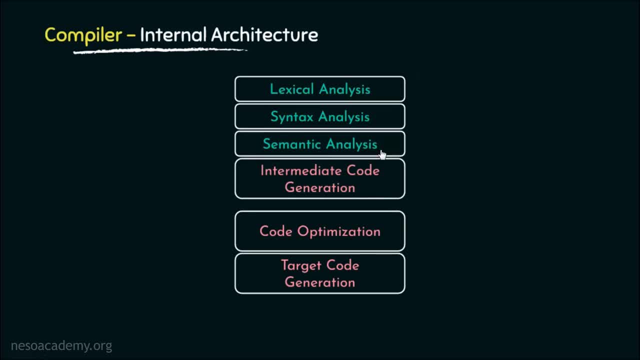 lexical, syntax and semantic analysis phases and, along with that, the intermediate code generation phase. these four are called the front-end, and the remaining two, ie the code optimization and the target code generation phase, are called the back-end. And why is so? 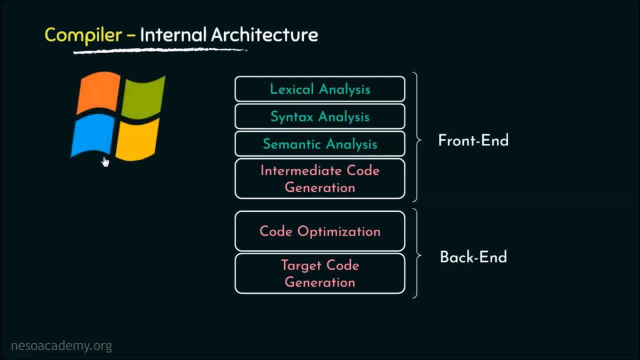 Suppose we have an existing C compiler for Windows platform. Now we would like to build a C compiler for a Mac operating system. For this we can modify the back-end, ie these two phases, according to the Mac specification and have those newly created back-end phases merged with the existing front-end and et. 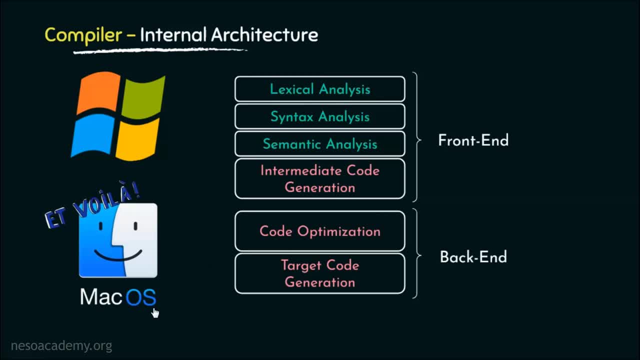 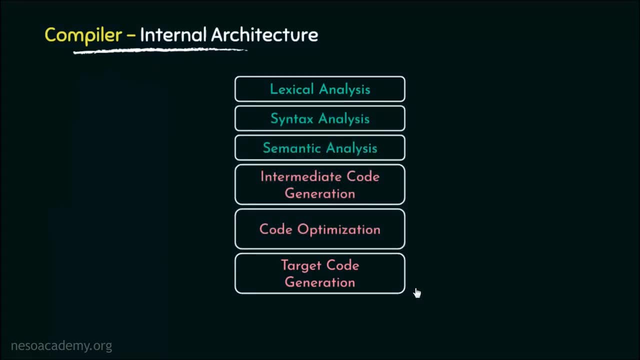 voila, We now have the C compiler for the Mac OS. Now, alongside these six phases, there are two more components of the compiler: The Symbol Table Manager And the Error Handler. Informations gathered from analysis phase are stored in the Symbol Table and used by 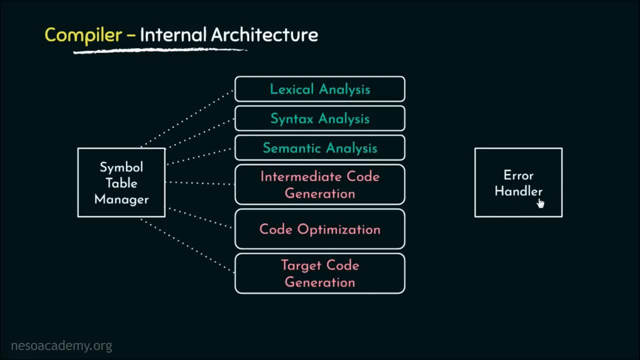 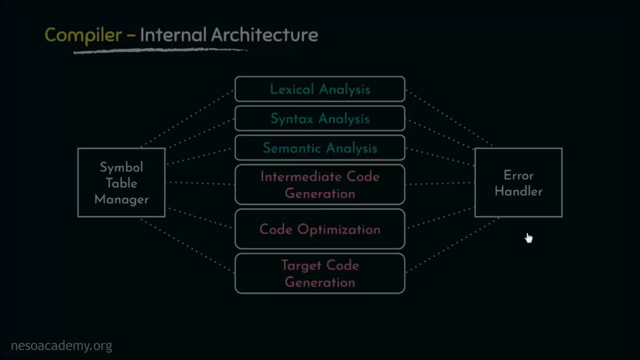 the Synthesis phase, And the Error Handler deals with the error detection and recovery. So these two are used by all the six phases. Now, in a nutshell, this is exactly the compiler design course. Now, if we talk about the course plan ie, the syllabus it is as follows: 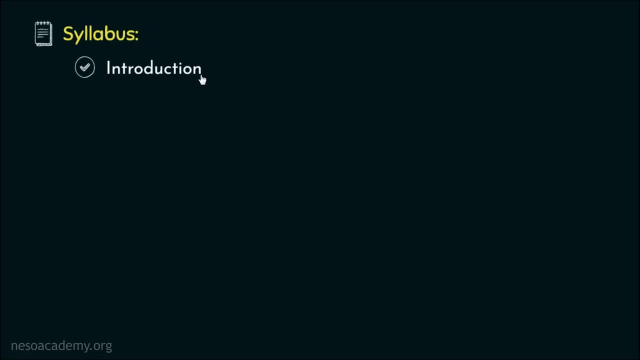 Chapter 1 will be the Introduction. Here we will cover the Symbol Table and the Lexical Analyzer. Chapter 2 will be the Syntax Analyzer. In this chapter we will get to know about different classifications of context-free grammars. Next up is the Top-Down Pursers. 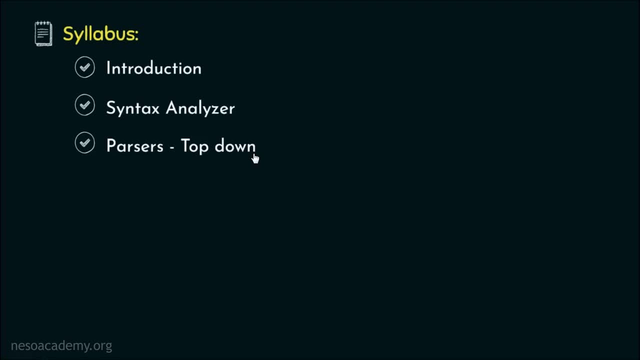 Here we will mainly focus on the Recursive, Descent and LL-1 Pursers. Also, while covering LL-1 Pursers, we will learn about First and Follow In Chapter 4.. We will learn about Variables. We will learn about various Bottom-Up Pursers in details. 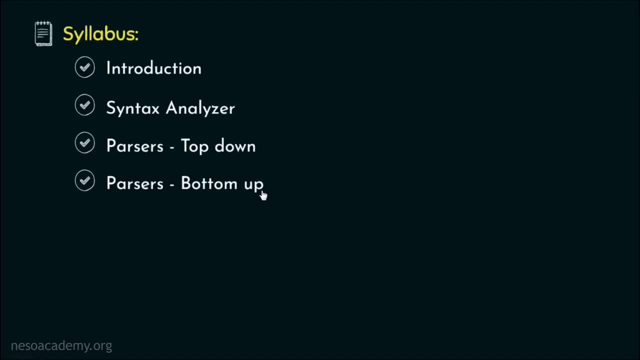 First we will study the most unique Purser, ie the Operator Precedence Purser, and thereafter we will learn about various LR Pursers. Next up is the SDTS or Syntax Directed Translation Schemes. This is basically the Semantic Analysis phase. 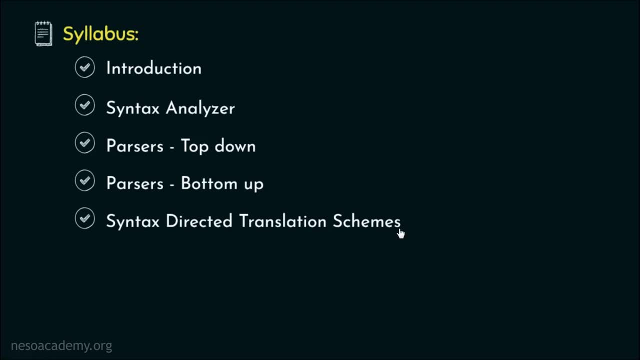 Here we will learn how the compiler looks for meaningfulness in our code. Now Chapter 6 will be all about Intermediate Pursers. Chapter 6 will be all about Intermediate Pursers. Here we will learn about the Intermediate Code Generation Phase. Intermediate codes can either have a linear form or a tree form. 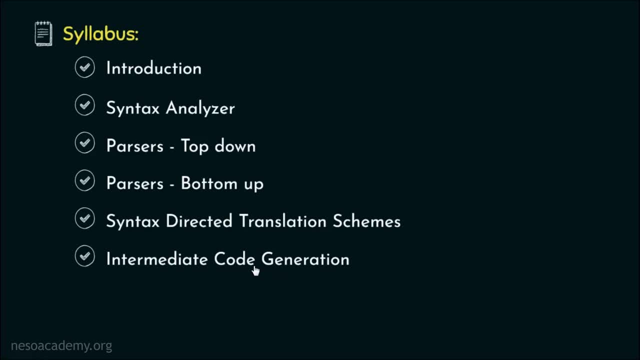 We will observe the very popular 3-address codes and the Directed Acyclic Graphs there. Finally, Chapter 7 will be all about Runtime Environment and Code Optimization phase. In Runtime Environment, we will get to know about the Process Structure in details and 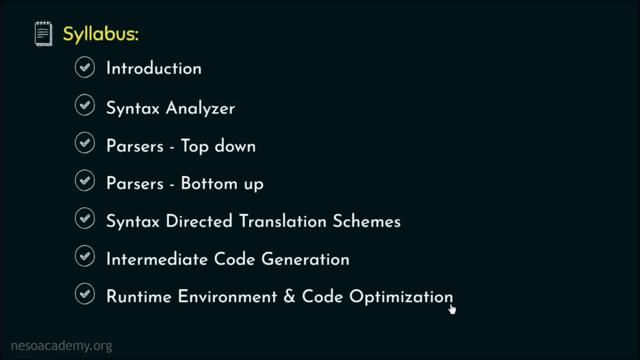 in Code Optimization phase we will observe the Process Forms in detail. In Code Optimization phase, we will observe the Process Structure in details. In Code Optimization phase, we will observe the Process Structure in details. will observe various machine independent and dependent code optimization techniques. 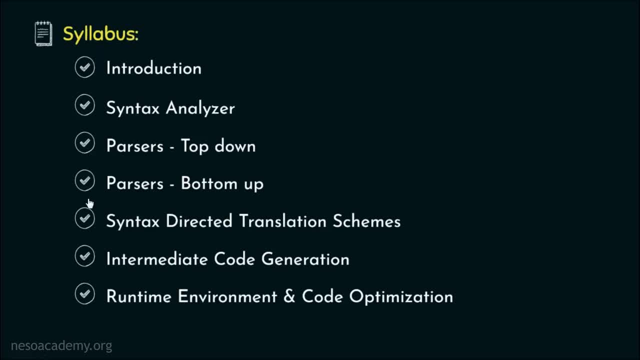 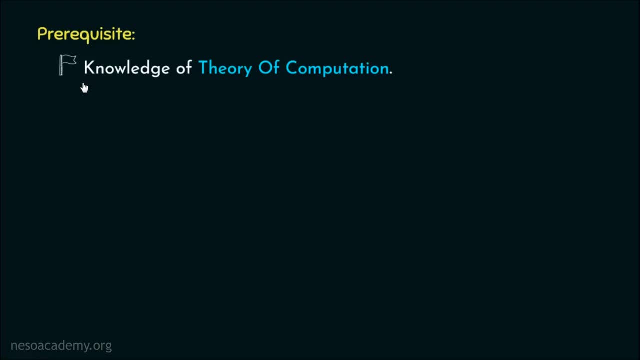 So, basically, our proposed syllabus will have seven different chapters. Now, since it is not a basic course, in order to study compiler design, the learners need to have a basic understanding of the subject Theory of Computation. So I strongly recommend you all to go through our beautifully presented Theory of Computation. 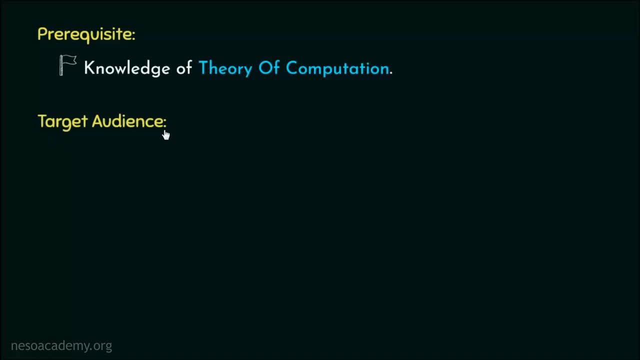 course. Now coming to the audience: whom keeping in mind this course has been designed? all the college and university students can take this course, because this course will be taught comprehensively. Next, any aspirant willing to take part in any competitive exam will be able to lucidly. 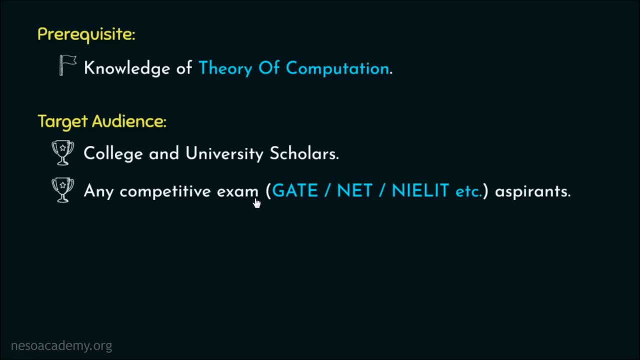 understand many numerical problems, along with the most apt illustration of the theory involved in those. Finally, any computer science admirer who just wants to get wise with the theory of computer science will be able to take part in this course. Now coming to the audience, whom keeping in mind this course has been designed? all the 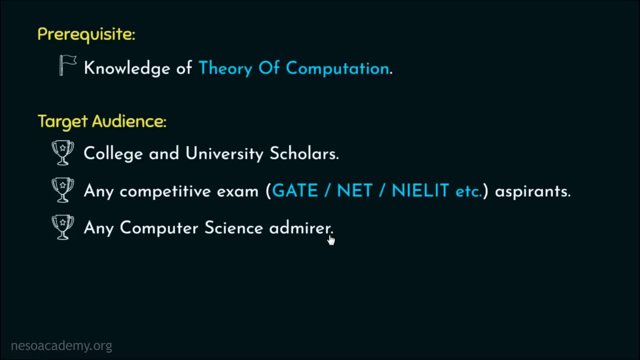 college and university students can take this course because this course will be taught comprehensively. Next, any aspirant willing to take part in any competitive exam will be able to lucidly understand many numerical problems, along with the most apt illustration of the theory involved. 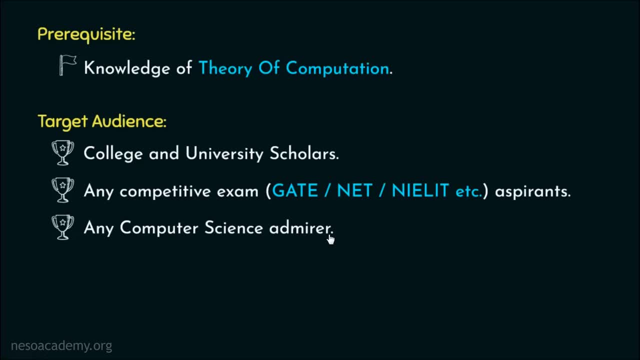 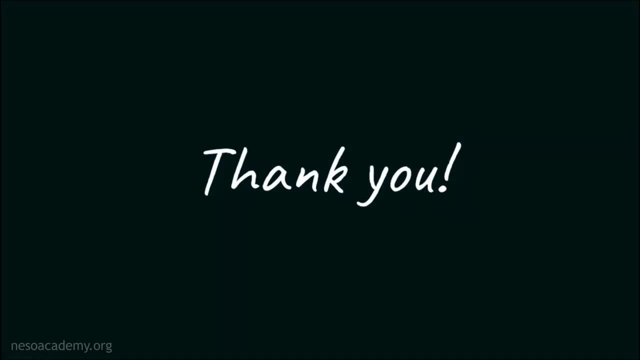 in those. Finally, any computer science admirer who just wants to get a quick detail recall about any topic of compiler design can refer to the lectures. Alright, people, That will be all for this session. In the next session we will observe all the phases of compiler with the help of a proper 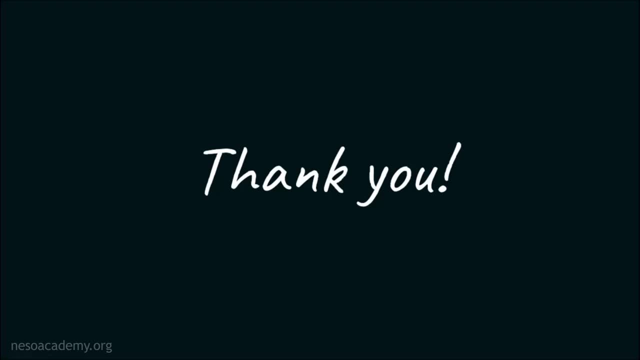 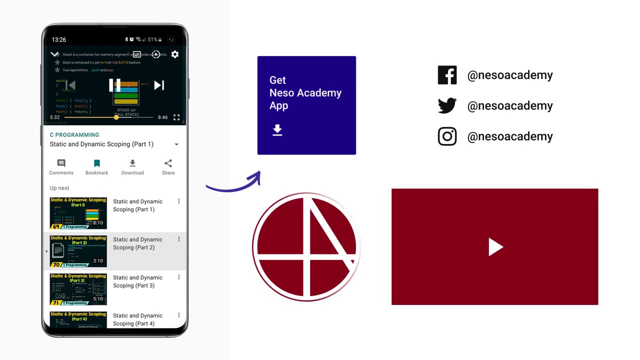 illustration, So I hope to see you in the next one. Thank you all for watching, Thank you.